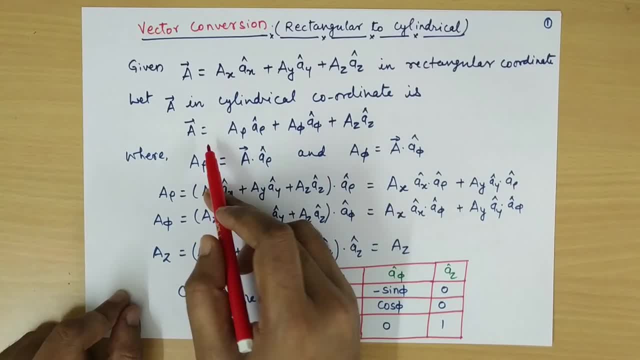 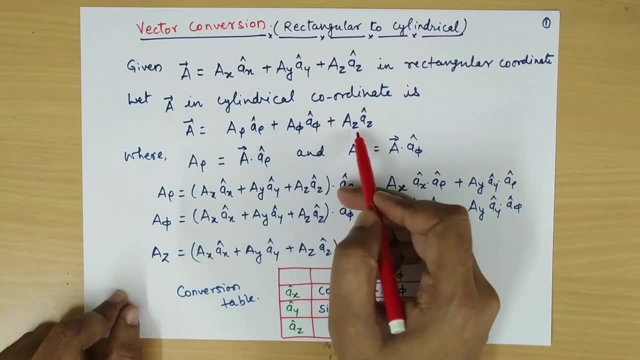 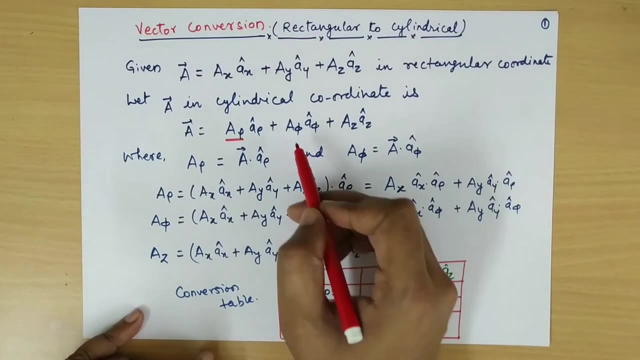 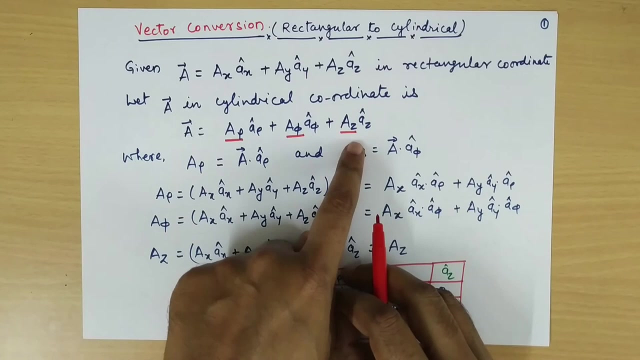 vector in form of cylindrical coordinate system as a equal to a rho, a rho, a phi in phi direction, az in z direction, where a rho is the magnitude in rho direction, a phi is magnitude in phi direction and az is magnitude in z direction. We can see that. 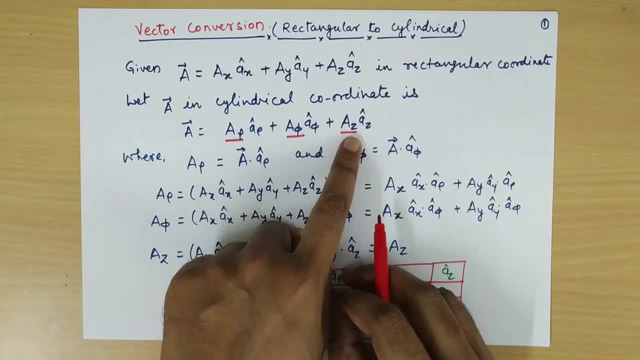 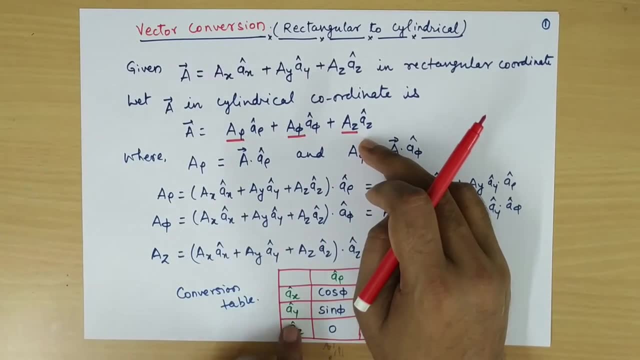 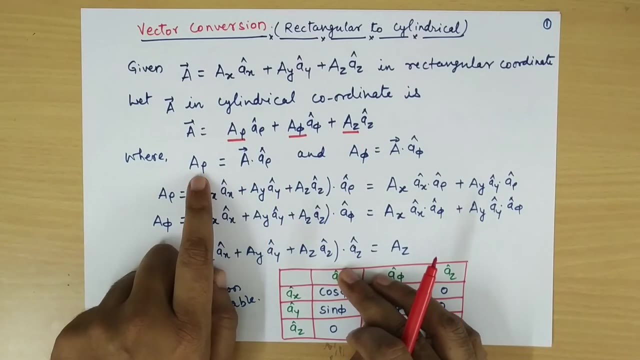 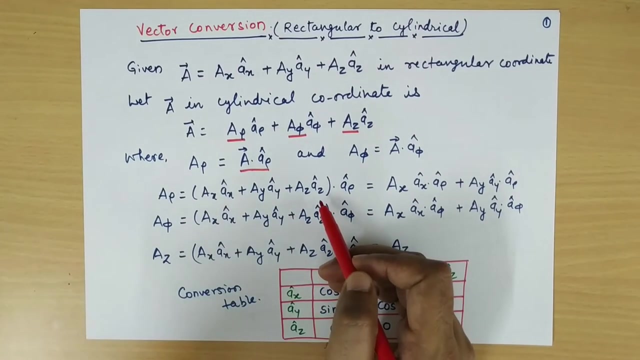 in z direction there will not be any change in the magnitude as we have the same value as in the rectangular coordinate system. but in and phi direction it is going to change. so to calculate that we have to calculate the arrow by using this so we can find a component of vector in any 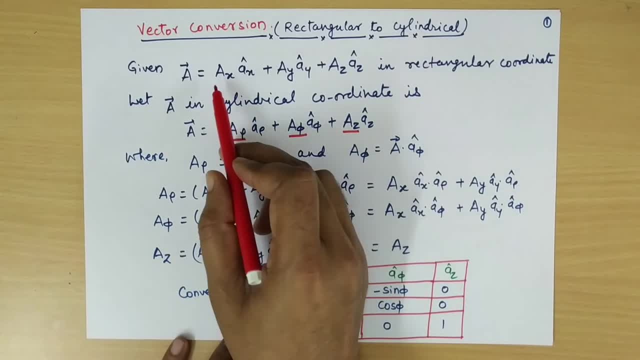 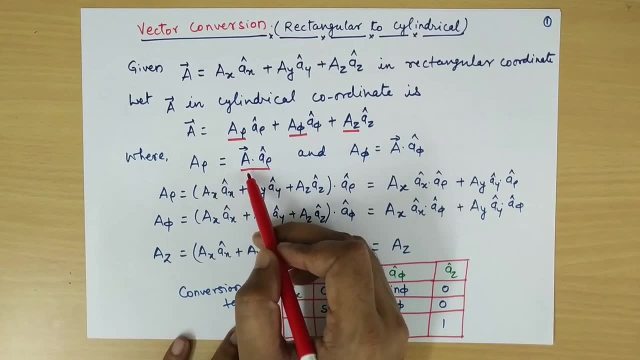 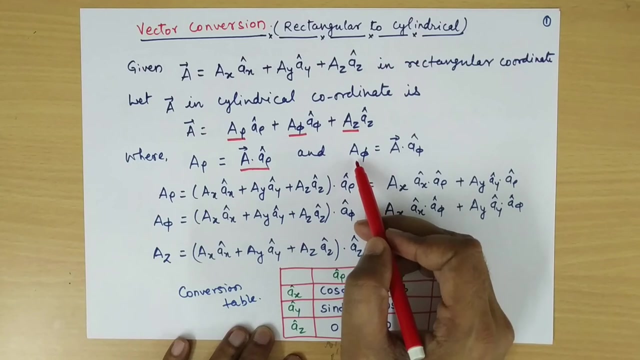 direction by taking the dot product of that vector with that direction. so here if I want to find component in row direction, I have to take dot product of this complete vector with arrow direction arrow unit vector. so it will be a dot arrow unit vector and for phi direction it will be a phi, which is a. 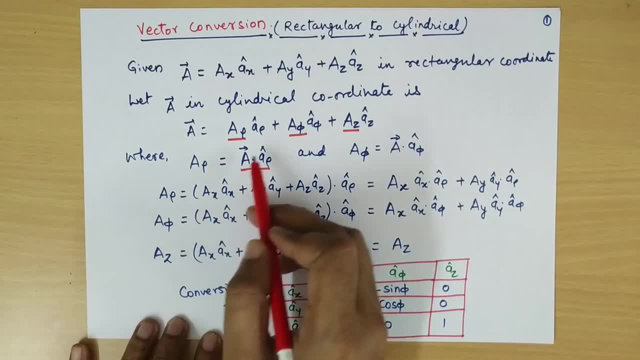 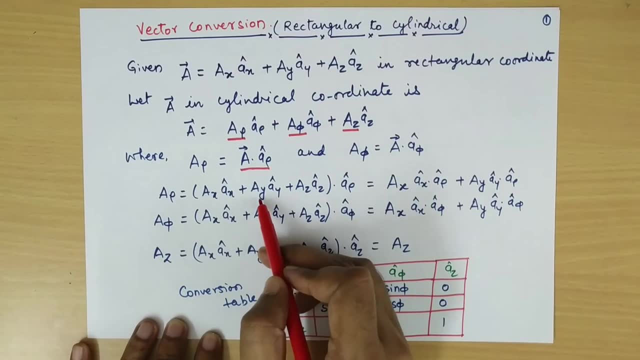 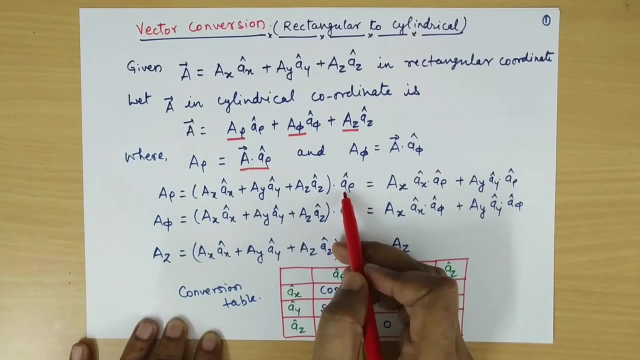 dot a phi direction. so when we apply this, what we found is when we apply this a here, ax, ay and az and take dot product with a dot product of this complete vector so we can find component of this with arrow, we will have ax dot arrow, ay dot arrow and az dot arrow in our 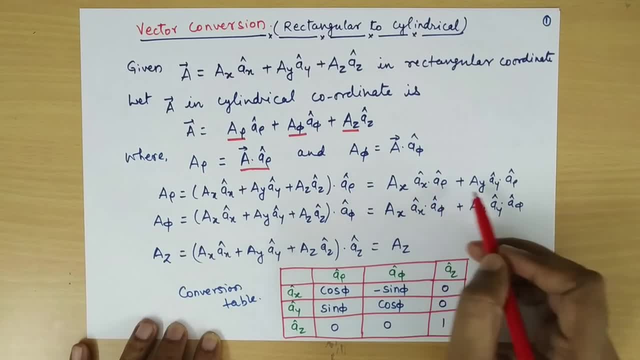 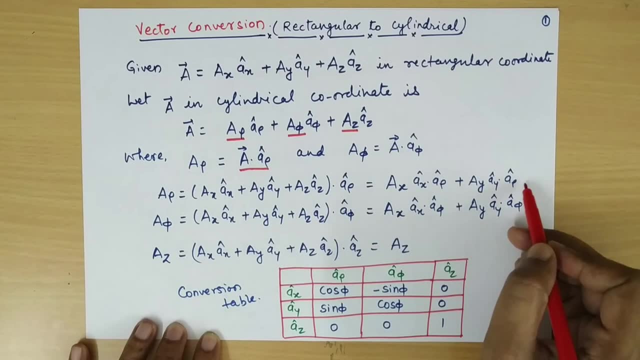 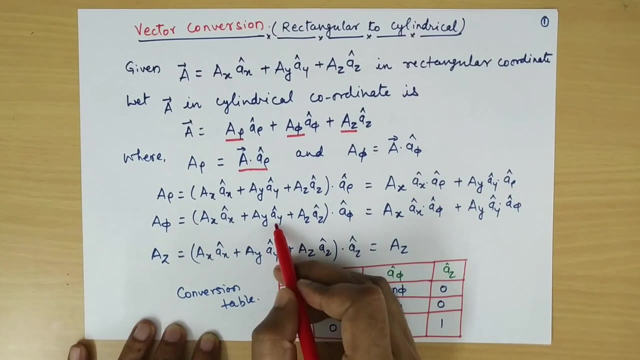 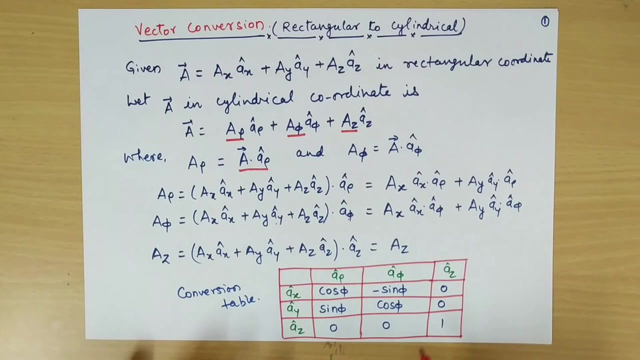 expressions. so ax dot arrow, ay dot arrow and az dot arrow, which ultimately going to be zero. that's why it is not shown here. similarly, for a phi it will be ax dot a phi, ay dot a phi and az dot a phi, which is again zero. so to make this conversion table, 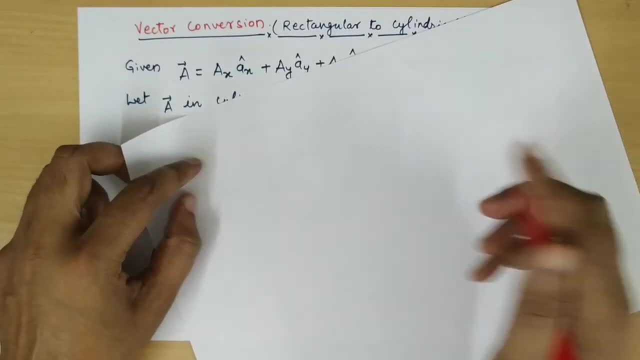 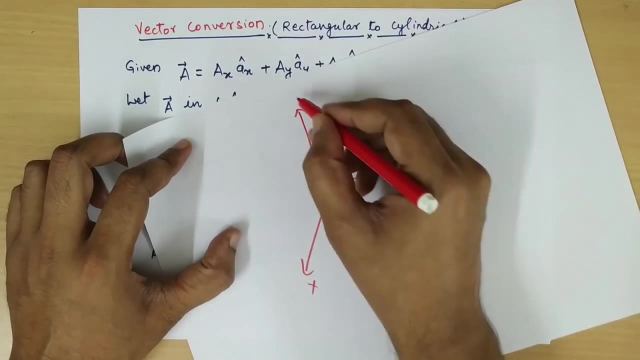 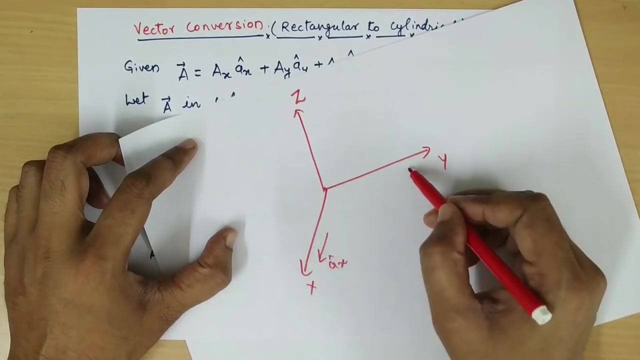 first of all, let us make the coordinate system in x, y and z direction, where this is the direction of unit vector ax, ay and az. now try to find the direction of x and y in first terms. take dot product equivalent of z and apply this with arrow. now try to find the direction of unit vector a, x, a, y and Z. direction in first terms checks and changes the positive position you are asking for the gradient between x and z and cube backward direction of the vector, unit vector and y and here on J onление. 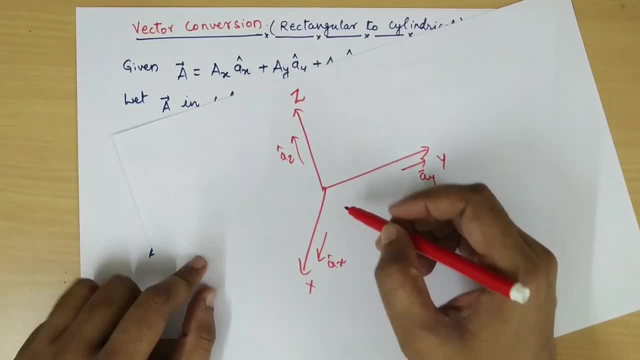 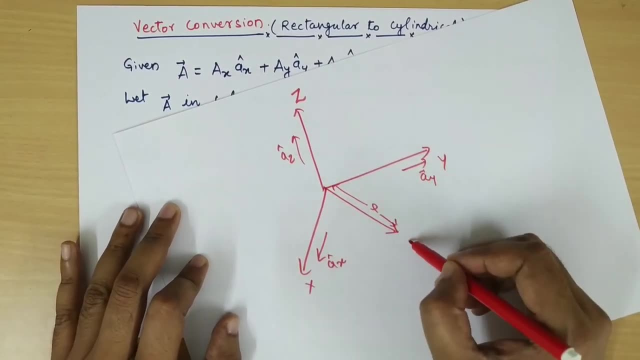 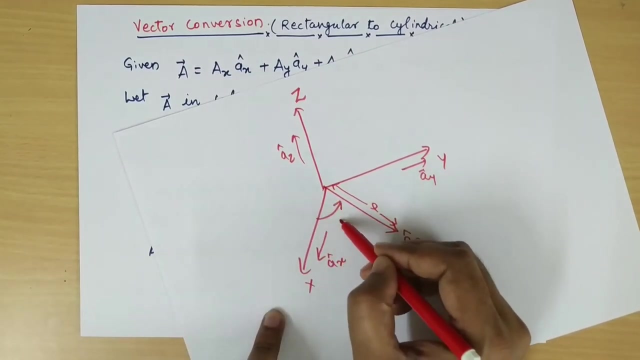 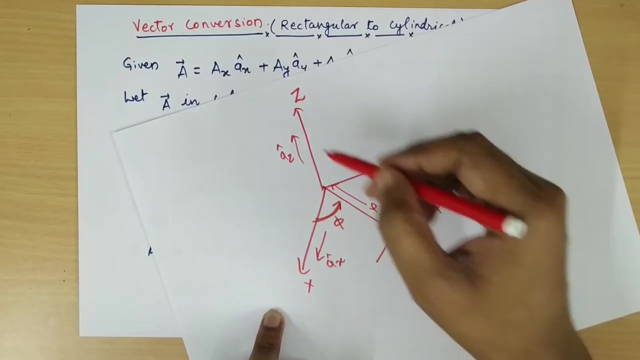 unit vector rho, phi and z. So for that the rho will be in this direction because this is rho, So the unit vector direction of a rho will be also same and phi is moving in this direction. So the a phi will be perpendicular to rho as well as z. that means a rho, a phi will be. 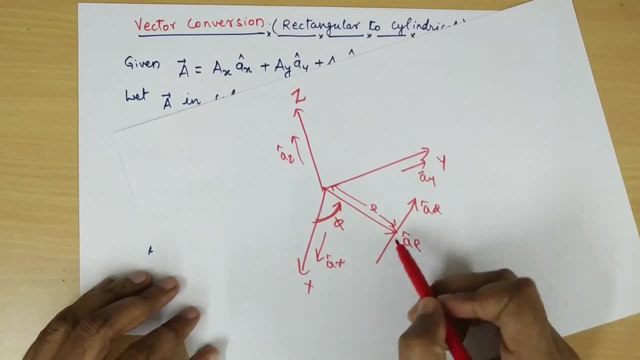 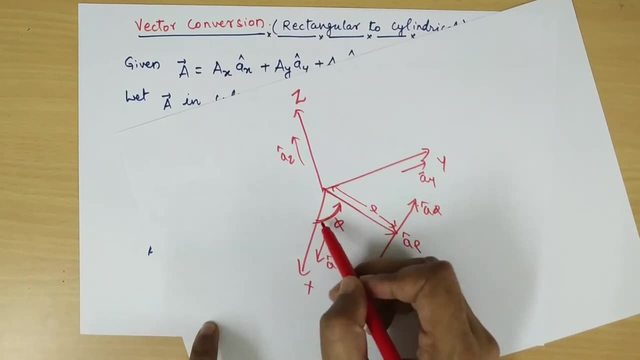 perpendicular to a z. So now find the relation between a rho and a x. So we can see a rho and a x. there is angle phi. So the dot product of a rho and a phi, a x and a rho, will be dot product. 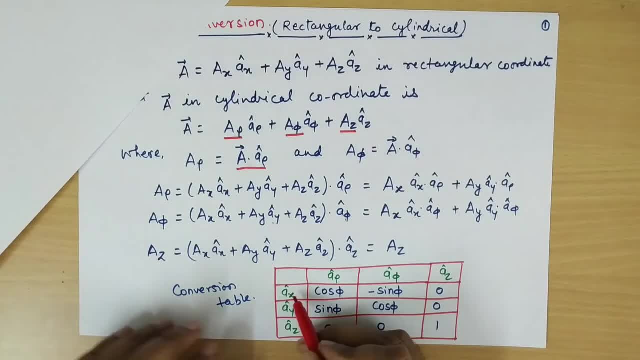 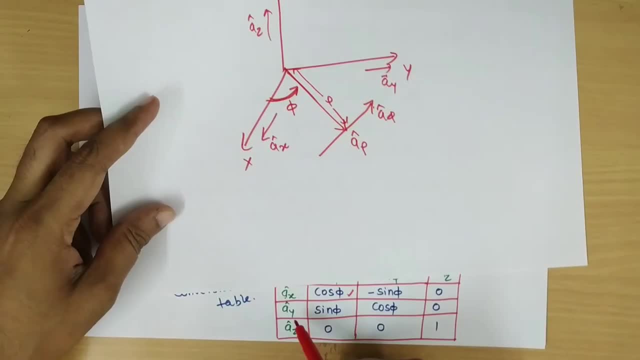 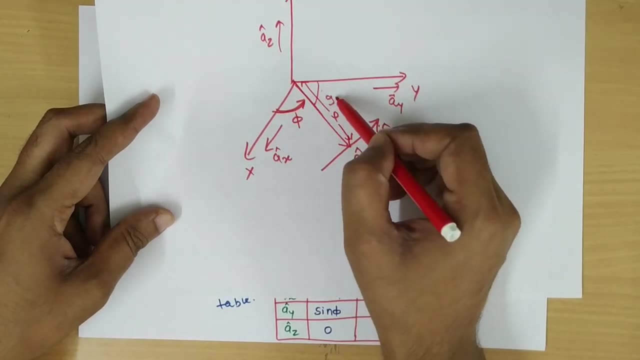 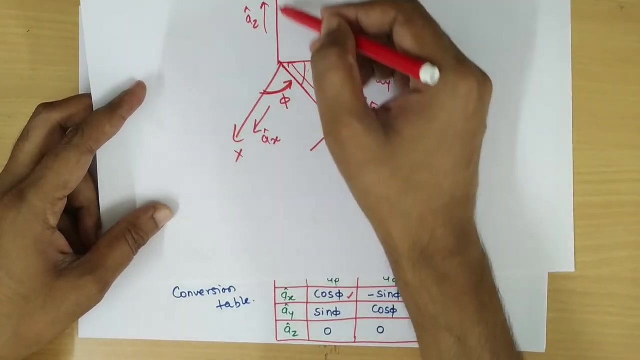 of a x and a rho will be cos phi, So dot product of a x and a rho is cos phi. Similarly, if we take dot product of this, a rho with a y, it will become sin phi, because the angle is 90 minus phi. So it will become sin phi. and if we take a rho and a z, the angle between this is: 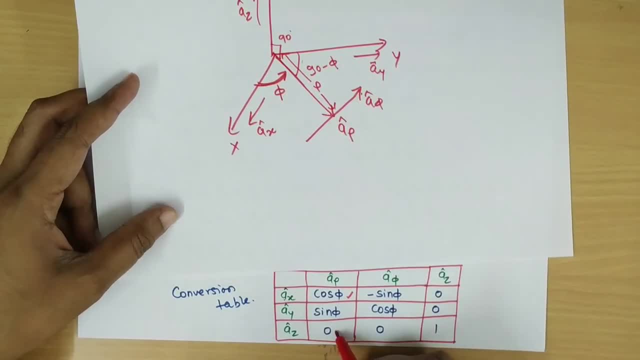 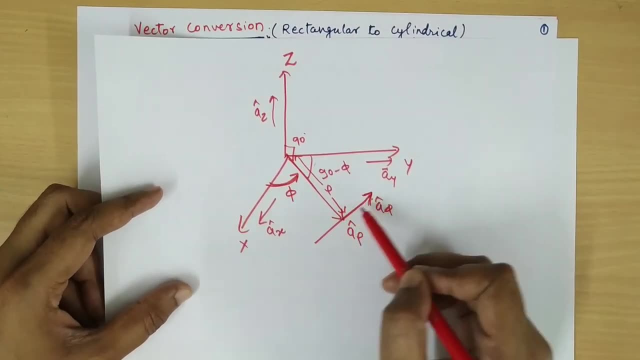 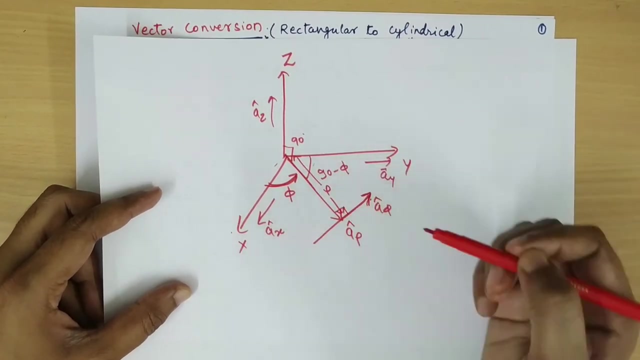 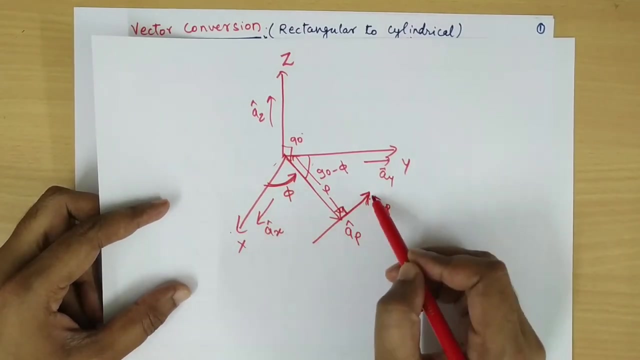 90 degree. hence the dot product will be 0.. Now to find the dot product between a phi and a x, we can use the angle as phi plus 90. So the angle is actually 90 plus phi between a x and a phi. 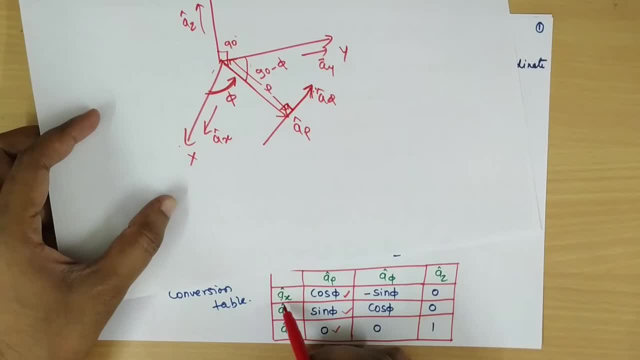 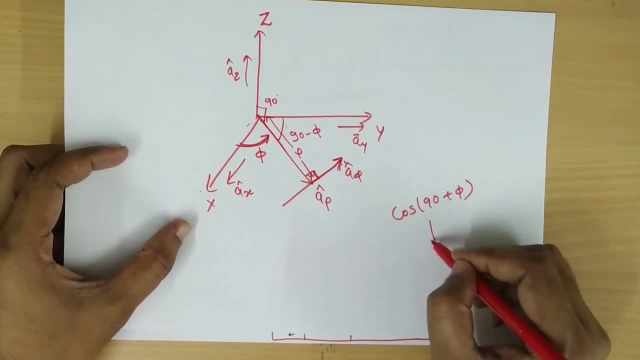 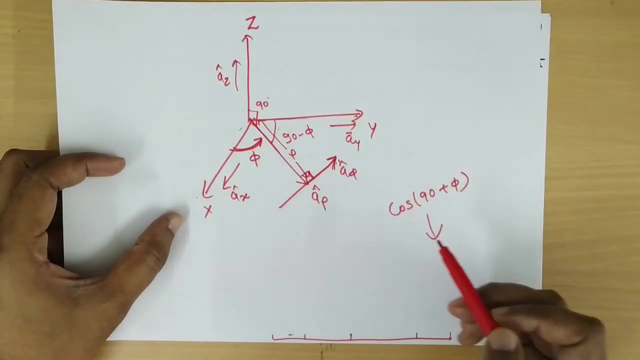 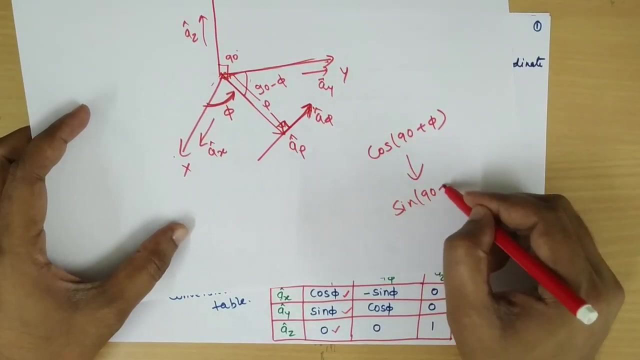 So if we take a x dot a phi, a x dot a phi, this will be cos 90 plus phi, which will be minus sin phi. Similarly, if I take a y and a phi, direction a y and a phi, So this will become sin 90 plus phi, because we have already. 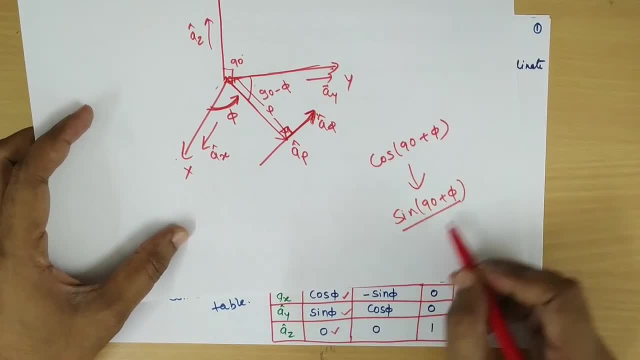 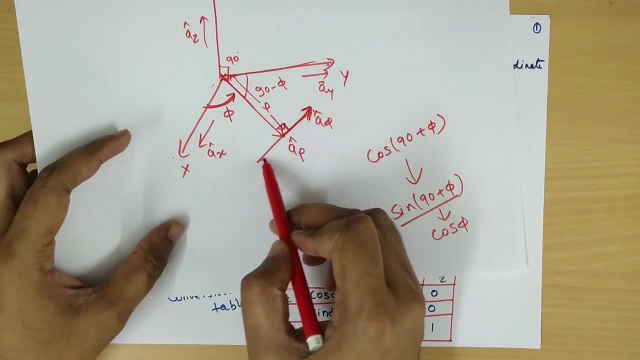 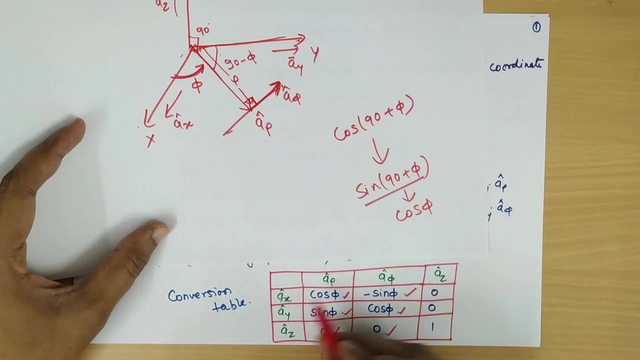 taken sin phi here, So here it will become sin 90 plus phi, and that is nothing but cos phi. this cos phi, and when we take this with z, z and phi is perpendicular to each other, So it is 0.. Similarly, for a z and a x dot, product of a z, a x is 0.. So if we take a y and a rho and a rho, 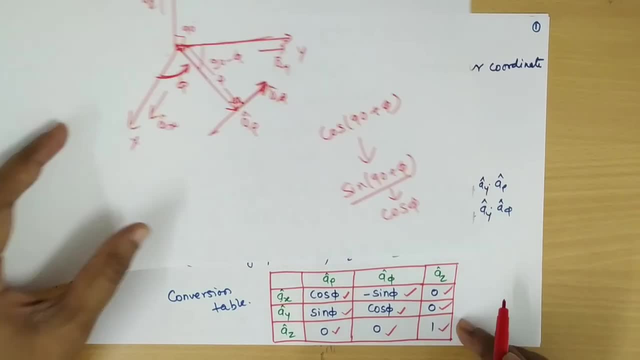 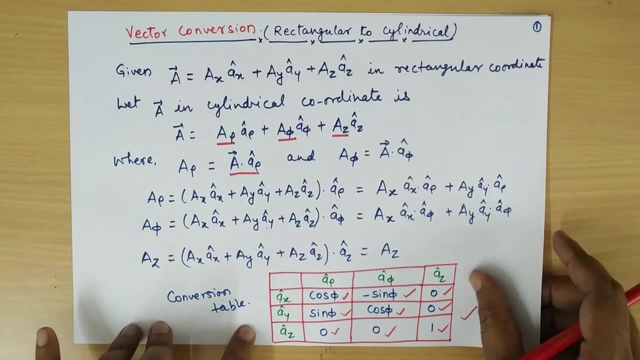 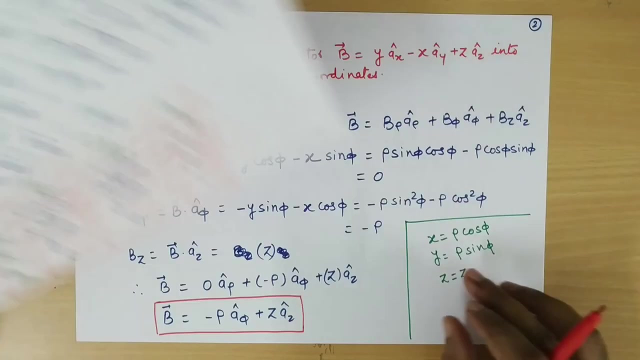 is 0.. So this is how we can find the conversion table, and this conversion table is very useful when we are converting from rectangular to cylindrical or cylindrical to rectangular. So let us take an example of this. So in this we have taken an a, vector b, which is y a x minus x. 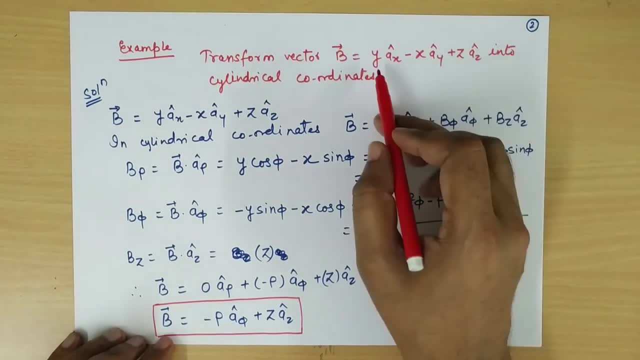 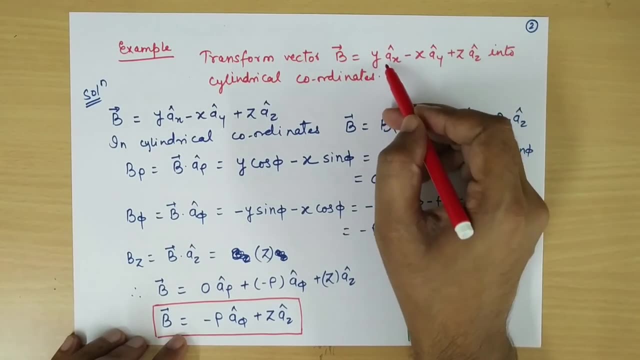 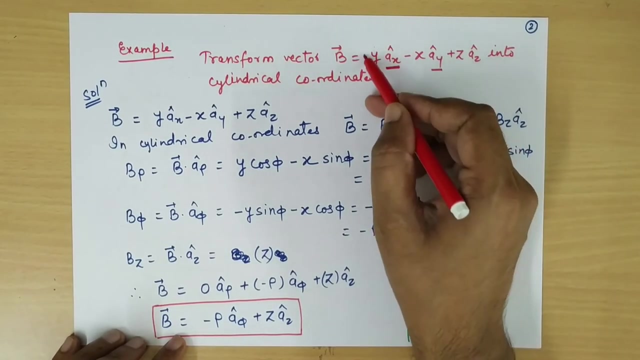 plus z a z and we have to convert this vector into cylindrical coordinate system. So remember, when it is asked to convert completely into cylindrical coordinate system, it means that the unit vector, as well as the variables which is used here, that is, y, x and z, should be converted. 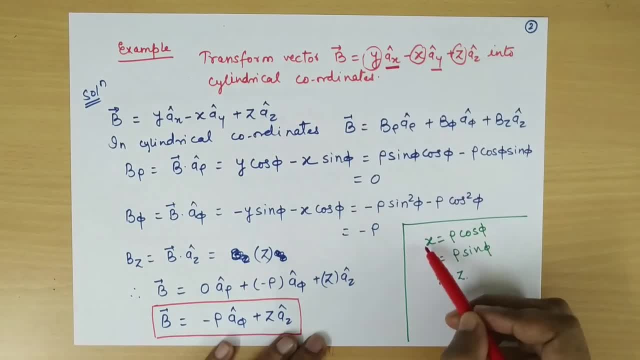 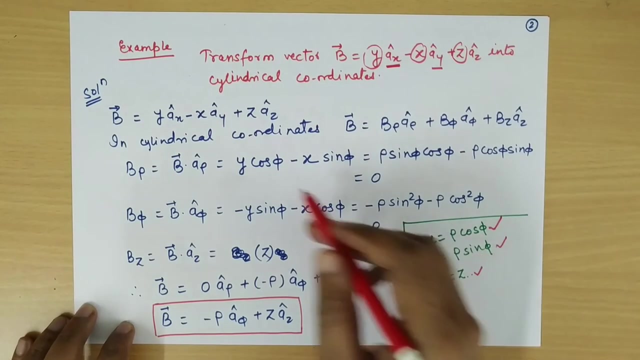 into cylindrical coordinate system and we know that x, in terms of cylindrical coordinate system, is rho cos phi and y is rho sin phi and z is same as z. so wherever we have x and y, we will be replacing with rho cos phi and rho sin phi in our calculations, and ax, ay and az. this will be: 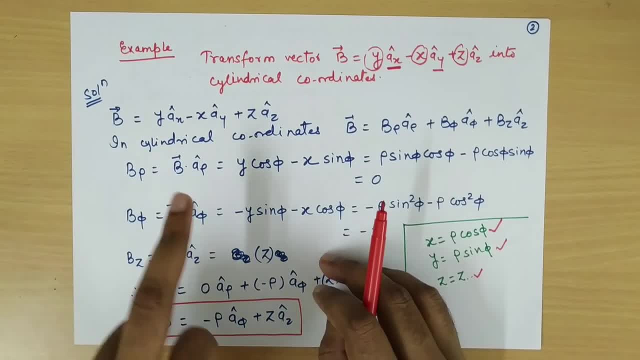 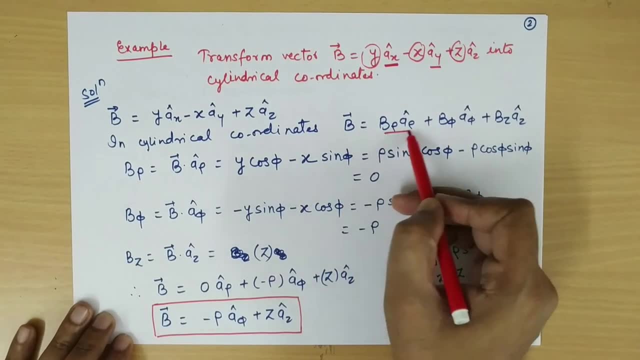 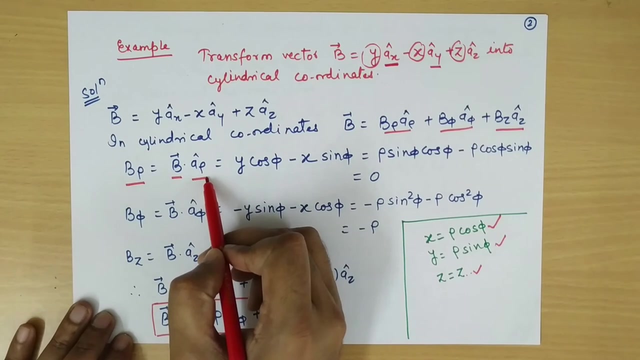 converted into cylindrical coordinate system. so first of all let us take b? rho, so b is b rho, a, b, phi a phi and b z a z. so b? rho will be dot product of b in the direction of rho, which is y cos phi minus x sin phi, so y. 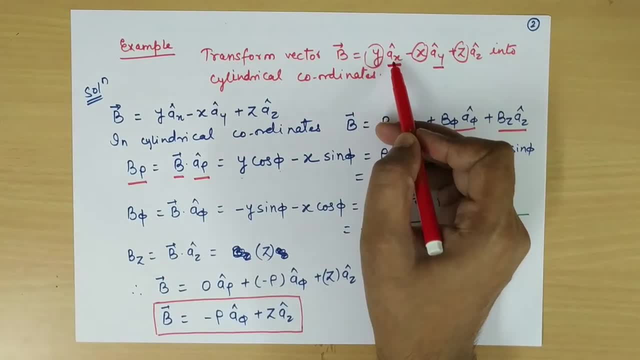 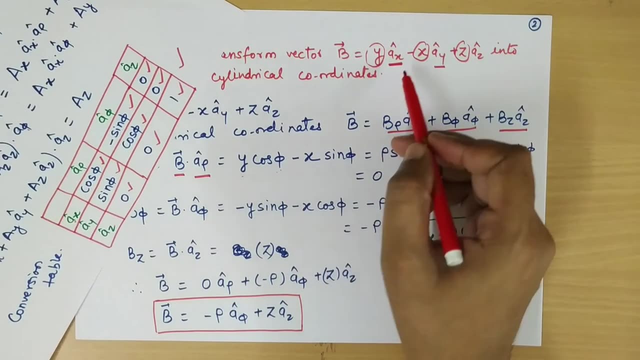 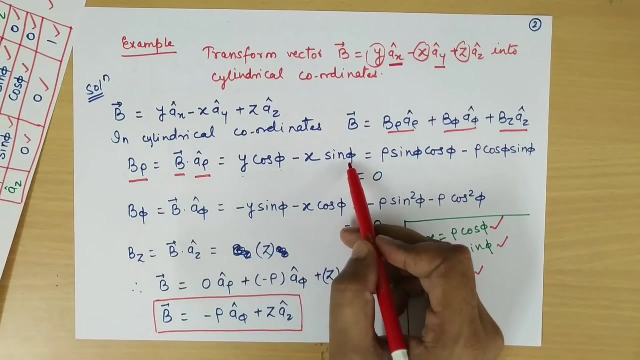 ax dot a rho. y ax dot a rho is cos phi. so we have taken that as cos phi and ay dot a rho. so ay dot a rho is sin phi. so this is y cos phi minus x sin phi. then y will be replaced by a dot product of b, dot product of b in the direction of rho. so y a x dot a rho is: 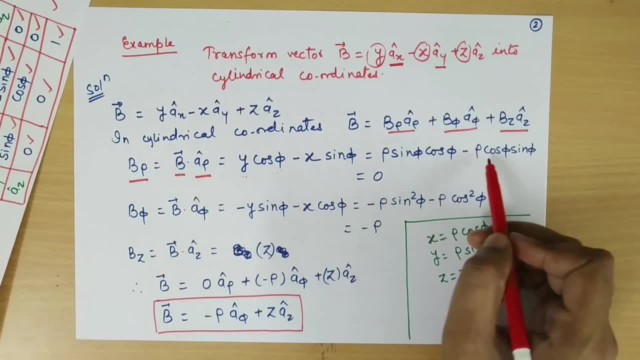 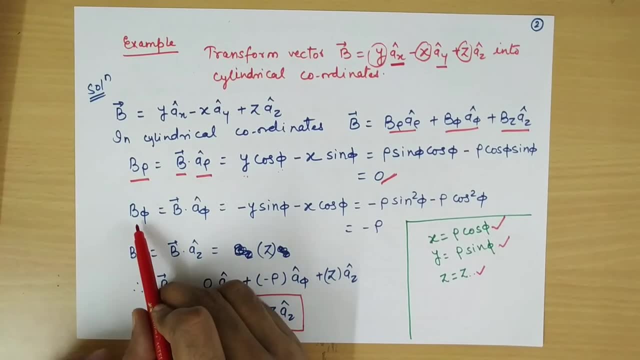 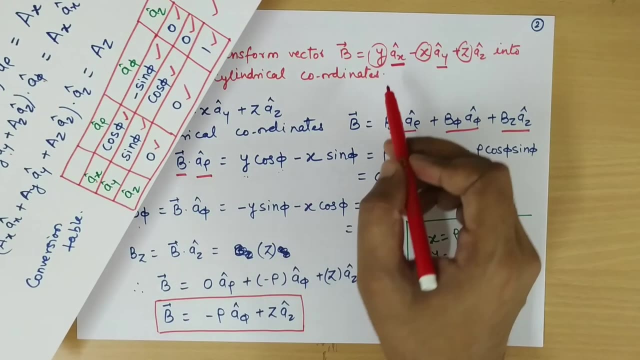 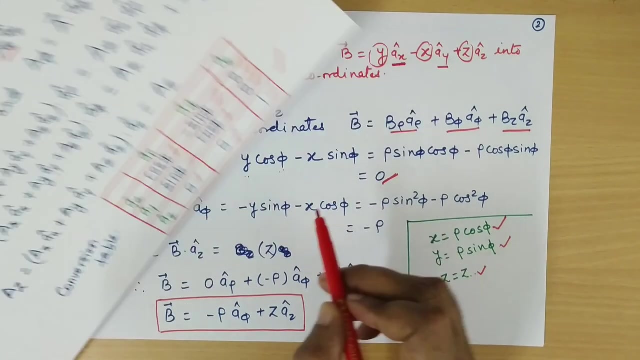 with rho sine phi here, and x is replaced with rho cos phi, and when we calculate we will get it as 0.. Then second one is b phi, so b dot a phi. b dot a phi means we are going to take dot product of a x with a phi, so a x dot a phi is minus sine phi, so it will give minus y sine phi. then we have: 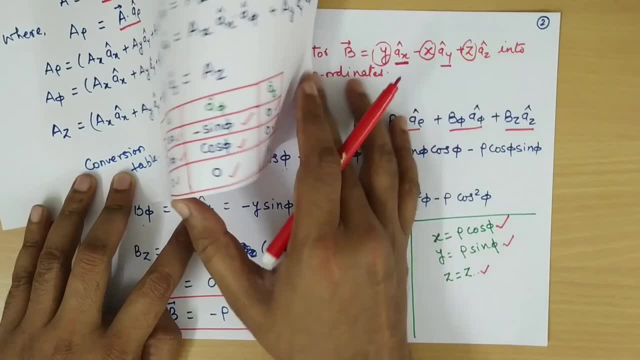 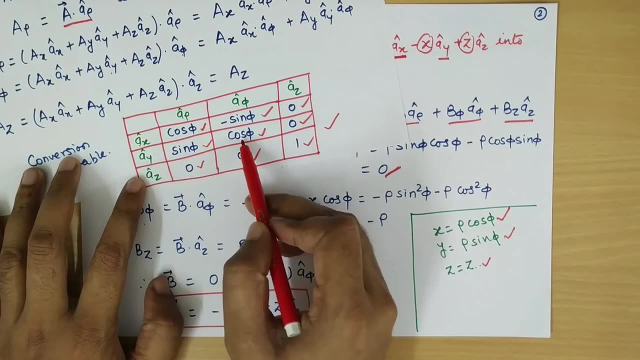 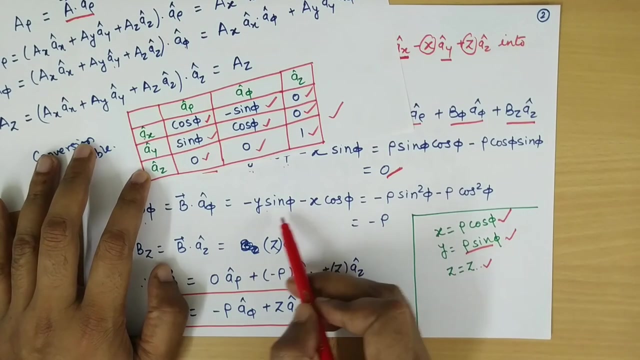 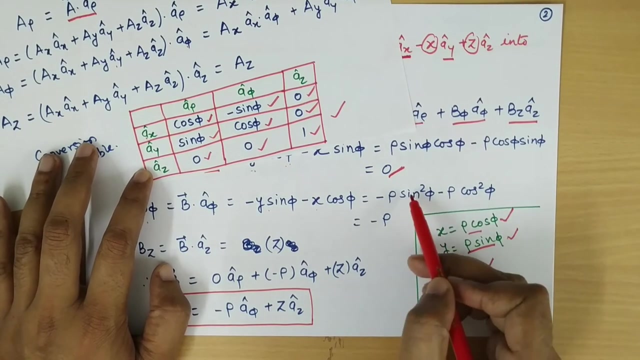 a phi. dot a y so a phi and dot a y so a phi. dot a y is cos phi. we can take minus x cos phi and by putting the value of y from here as rho sine phi and x as rho cos phi, we can find as minus rho sine square phi, minus rho cos square phi. 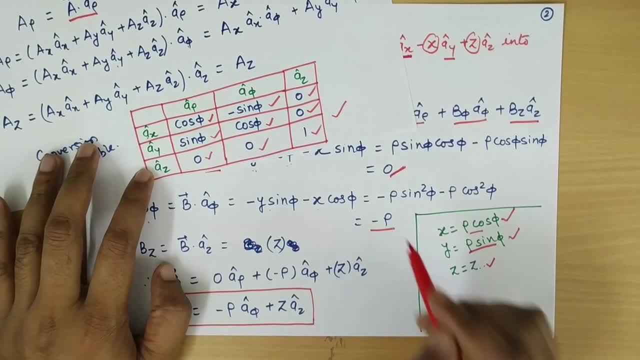 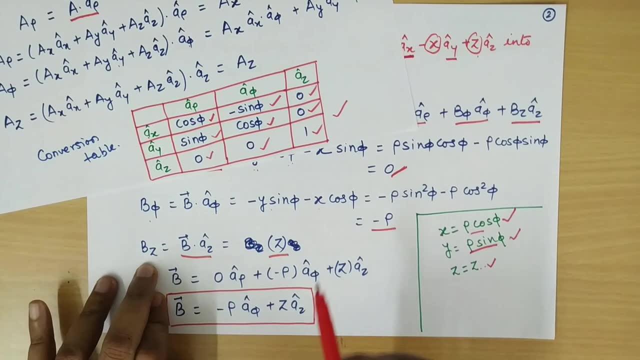 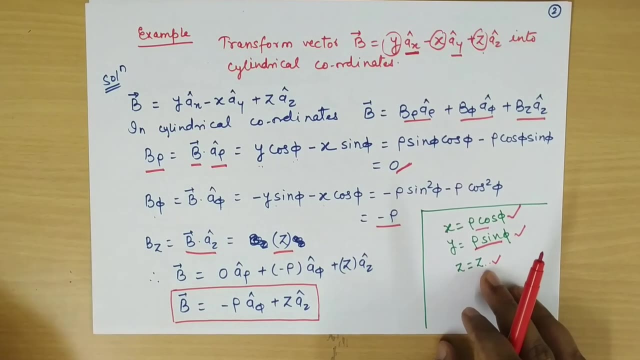 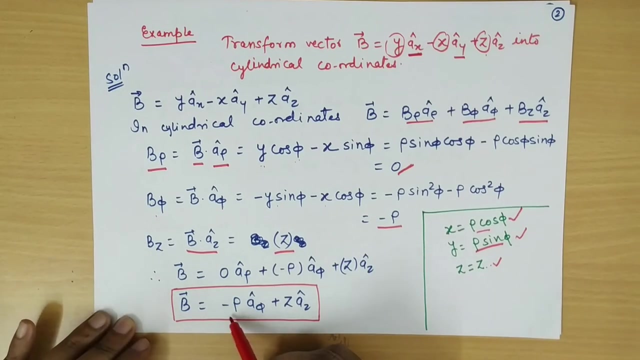 so sine square phi plus cos square phi is 1, it will become minus rho. b. z will remain same. that is already z. so if we take dot product we will again get z. so the vector will be b equal to 0, a rho plus minus rho. a phi plus z a z, so b is 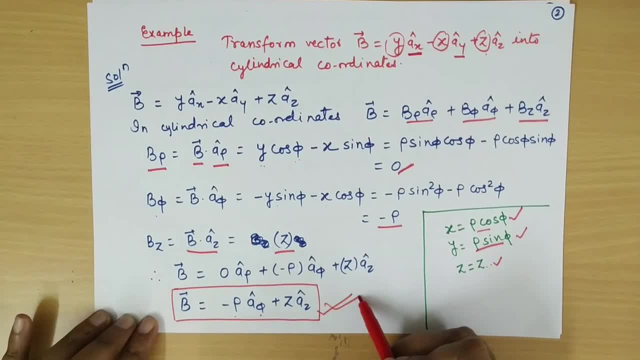 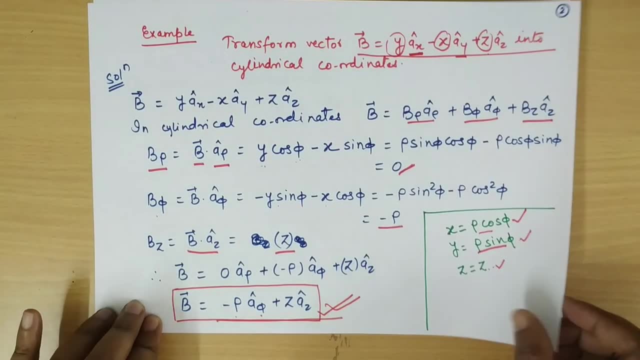 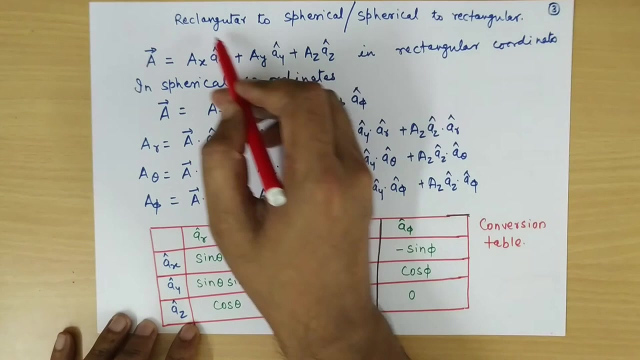 minus rho a phi, plus z a z. This is our converted vector from the rectangular coordinate system to cylindrical coordinate system. Next we are going to study about conversion from rectangular to a spherical or a spherical to rectangular. So this conversion can be done. 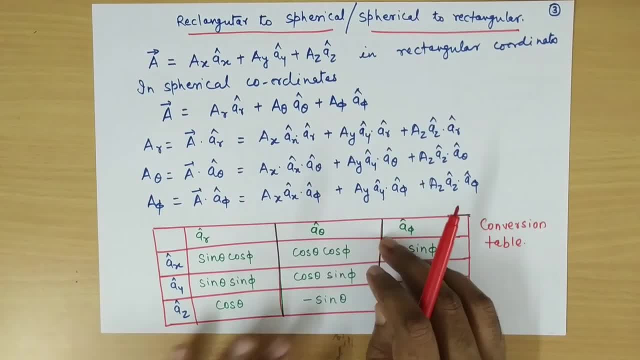 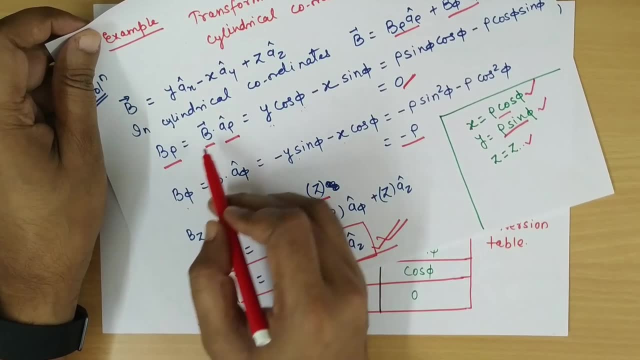 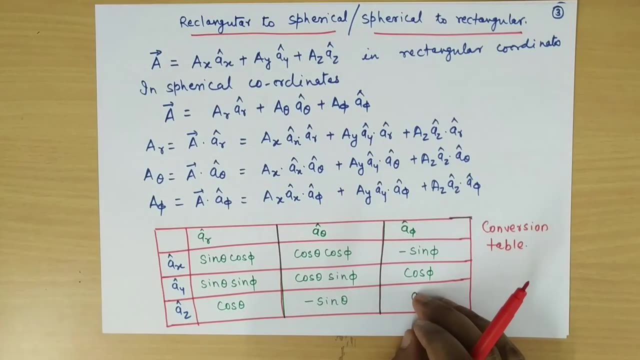 in both the way. Suppose we have been given with rectangular coordinate system. Again we will do the same thing to find b, x. we can take b dot a x, So that way we can calculate the. we can convert cylindrical to rectangular. Here, to convert rectangular to a spherical, 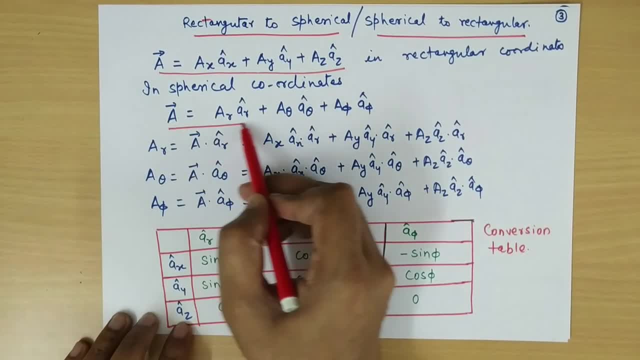 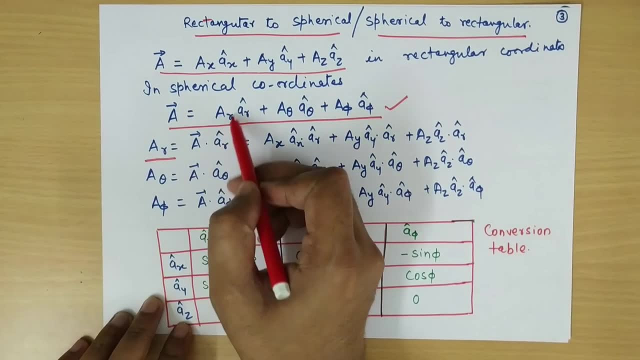 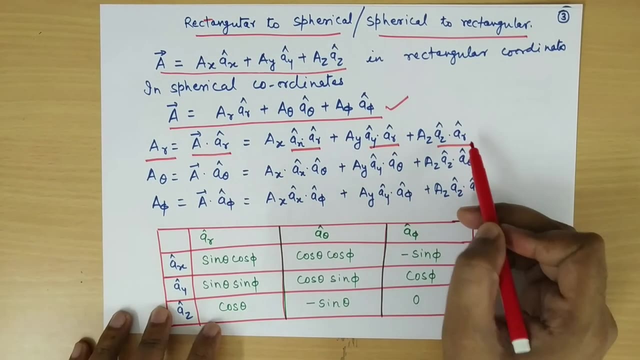 we will take a vector and write the form, a spherical form of this, And take the component in r direction. that is a dot a r. So it will have a x dot a r, a y dot a r and a z dot a r. Similarly, when 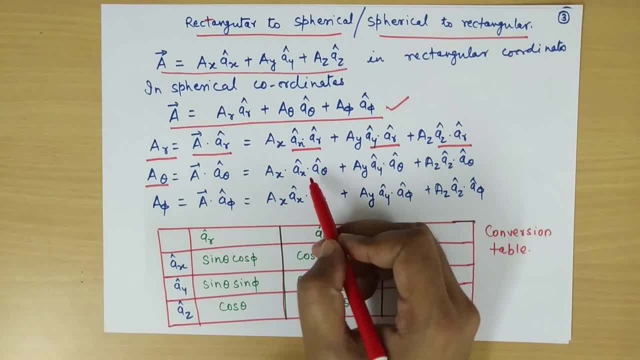 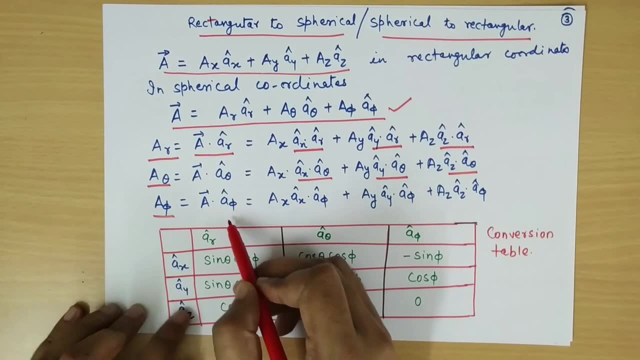 we take component in the direction of theta. we have a x dot a theta, a y dot a theta and a z dot a theta. In phi direction we have a x dot a phi, a y dot a phi and a z. 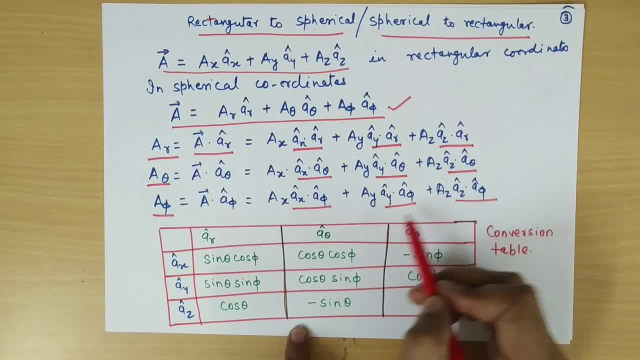 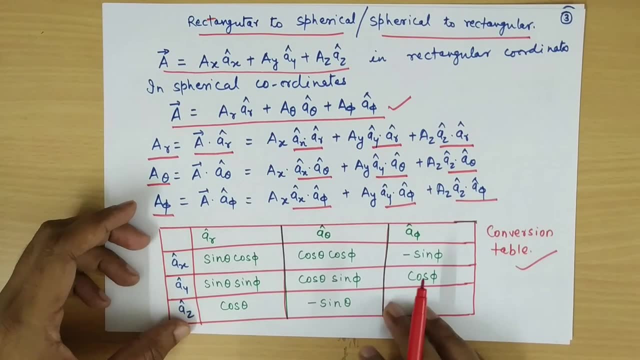 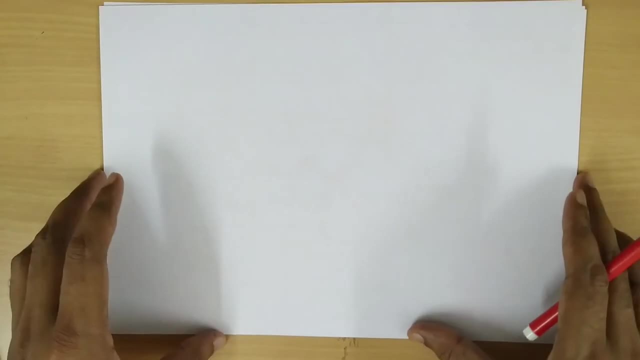 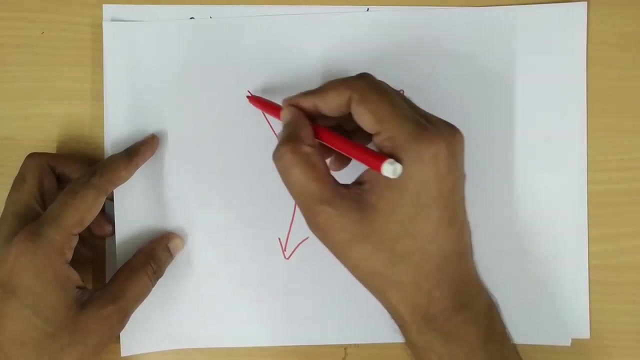 dot a phi. So we are going to calculate these all dot products and we will form a table which is known as conversion table, from rectangular to a spherical or a spherical to a rectangular. so to calculate that, let us make the coordinates system again. so let's say this is X, Y and Z, as we know. 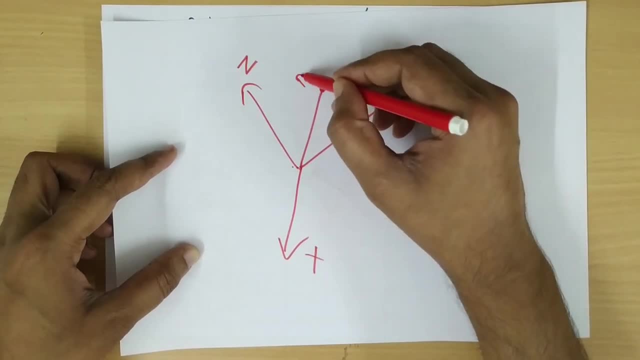 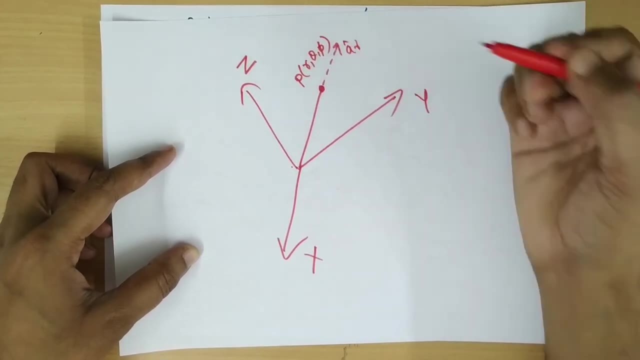 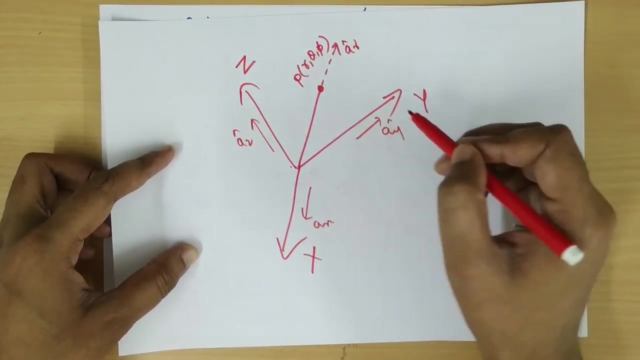 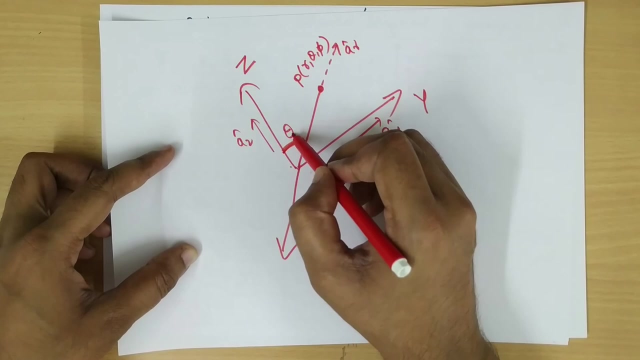 that this point is, let's say, P, which is r, theta of I. so the direction of a are will be this and a z direction is this. this is Ax and A1. so to find dot product between a, Z and a are, the angle between. this is defined as theta, so this will be. 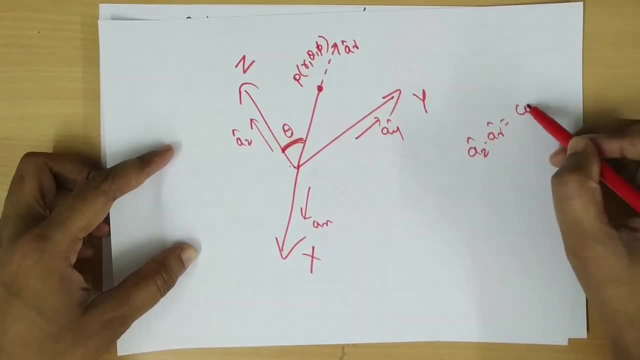 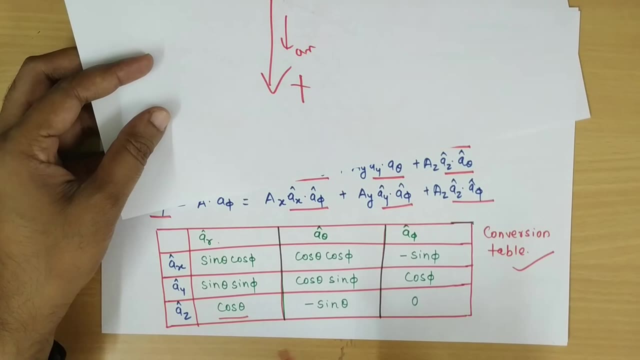 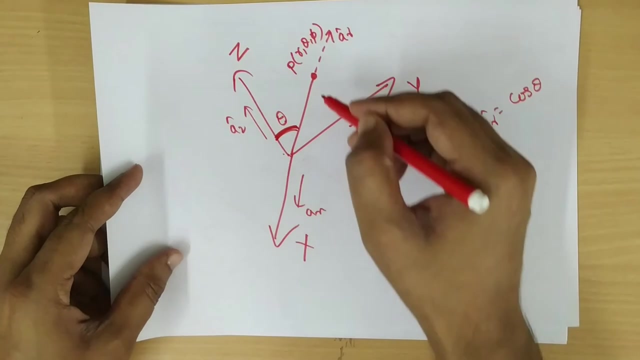 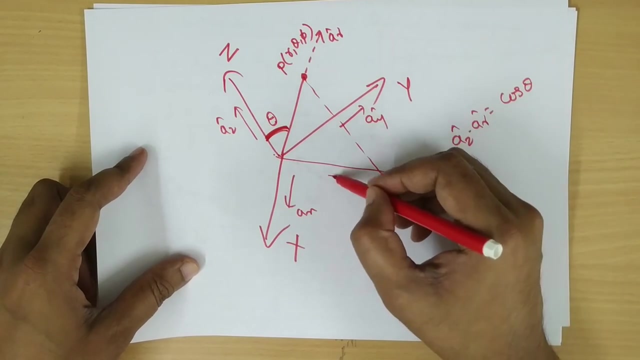 a Z, dot a R will be theta because angle between these two. so we can see: AZ and AR is cos theta. now next is AY and AR, AX and AR. so for AX and AR we will take the projection on XY plane. so this projection is nothing but R sine theta. so this projection is R. 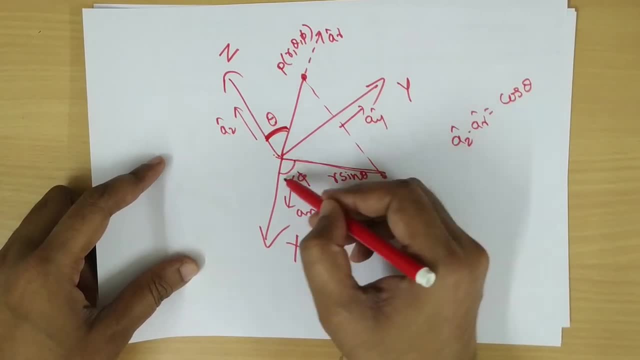 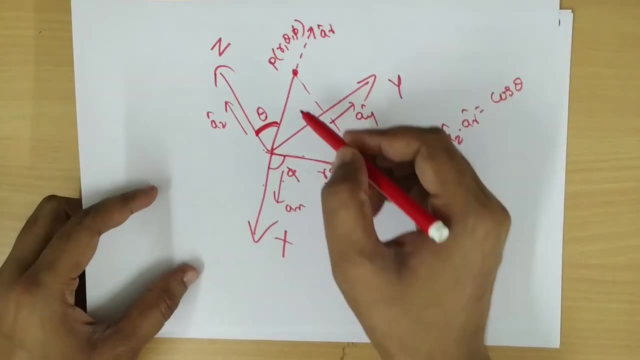 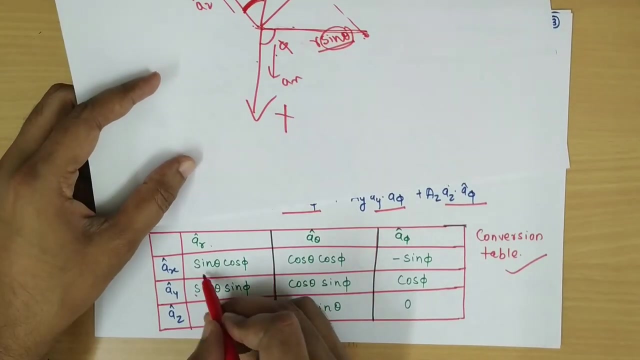 sine theta and this angle is Phi. so in between X and this projection it will be cos Phi, so R sine theta, cos Phi, when we are just converting it. so the angle between these two will be sine theta and cos Phi, so it's sine theta, cos Phi. 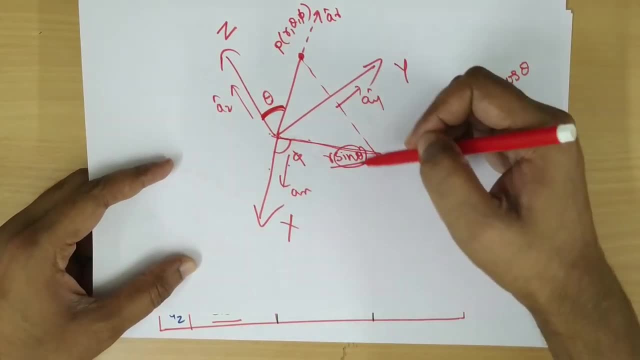 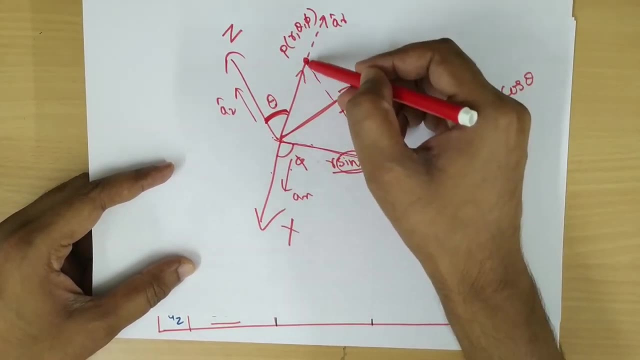 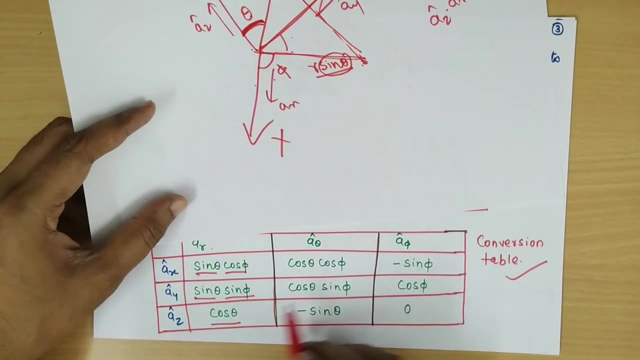 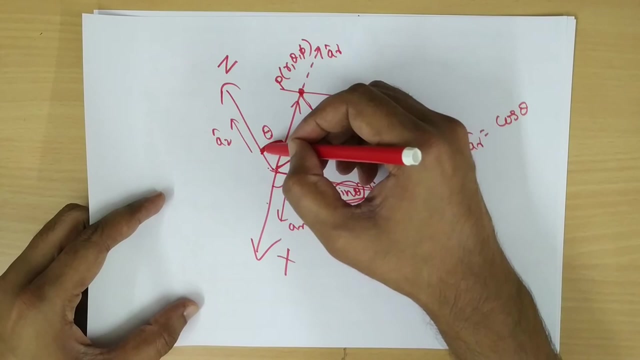 similarly, when we take the unit vector in the direction of Y and AX, then AR projection will be sine theta and then sine Phi. so it will be sine theta, sine Phi. same way we can calculate for theta direction. theta direction is 90 degree more than this AR direction. AR is theta, then this is 90 degree, so this: 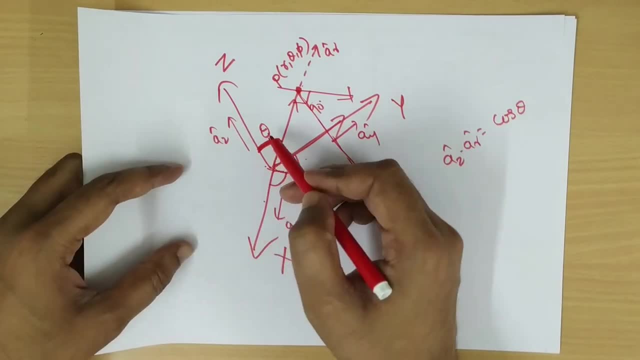 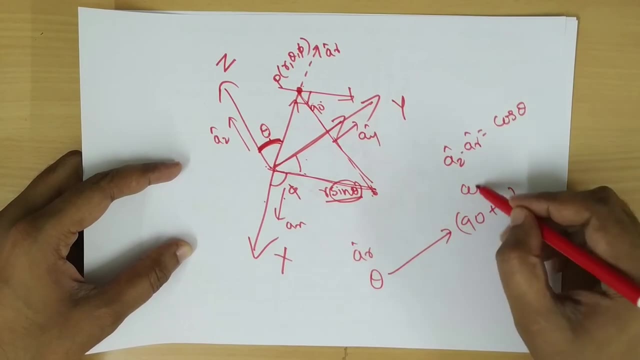 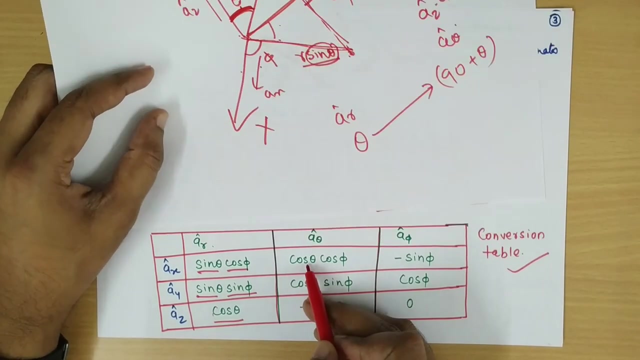 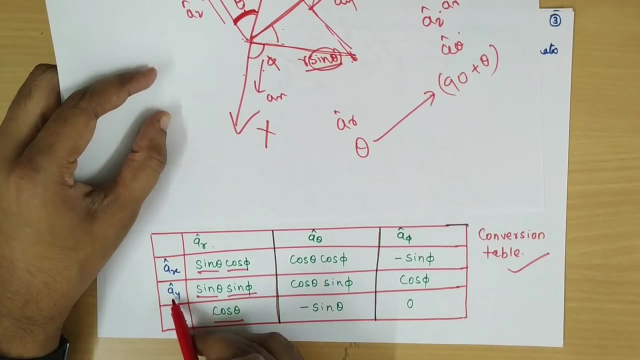 will become 90 plus theta. so wherever we have theta, if we just replace that theta with 90 plus theta, we can convert from AR to AX theta. so here this theta sine 90 plus theta is cos theta, so AX dot a theta will become cos theta, cos Phi. here sine 90 plus theta is cos theta, so AY dot a theta. 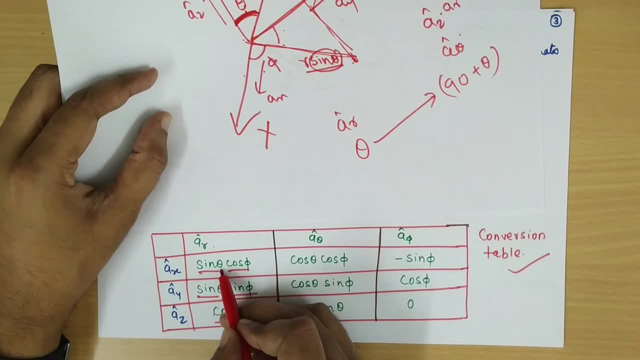 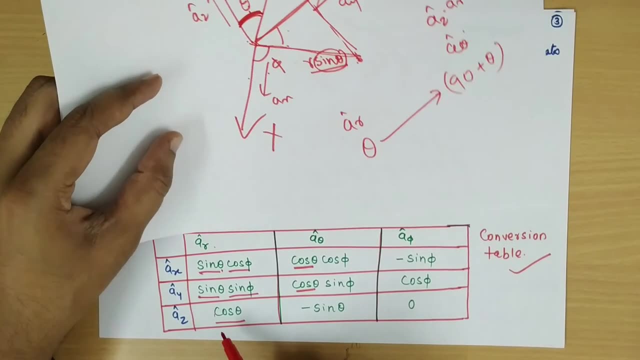 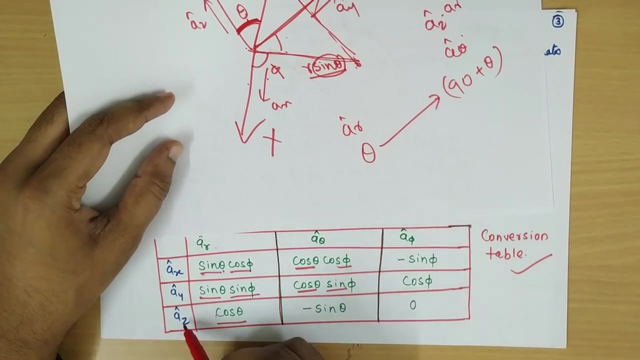 will become cos theta sine Phi. so in place of theta just write 90 plus theta to get these two terms. remaining terms will remain same. so this 5 completed now the angle between a theta and AZ. so here also in place of theta, if I write 90 plus. 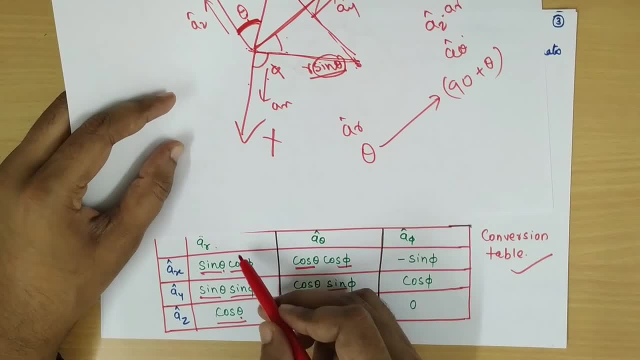 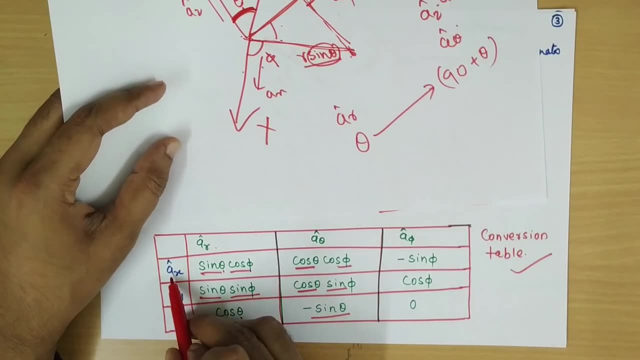 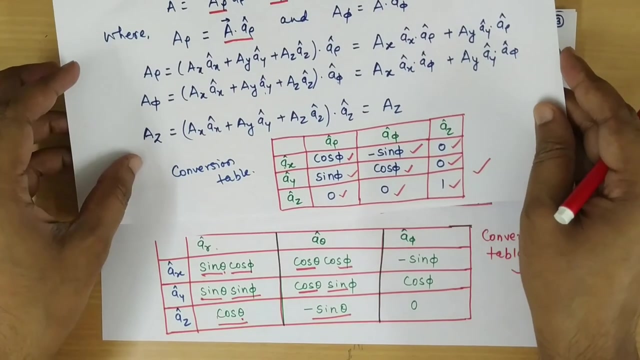 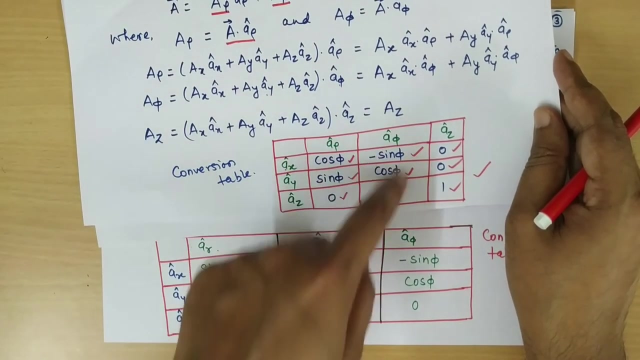 theta. so cos 90 plus theta is minus sine theta. so this is how we can write first column and then the second column. for third column we have to know angle between X and Phi, which was already done in case of cylindrical coordinate system. so when we write AX, AY, AZ with A Phi, so this: 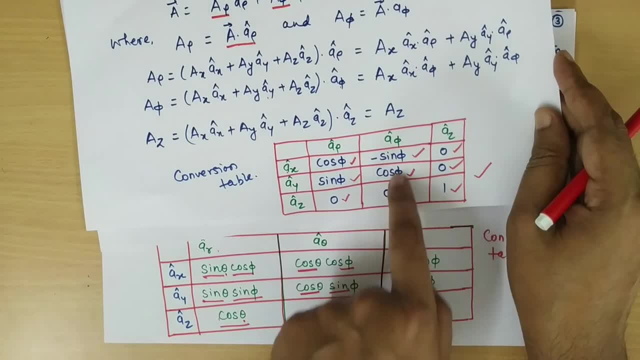 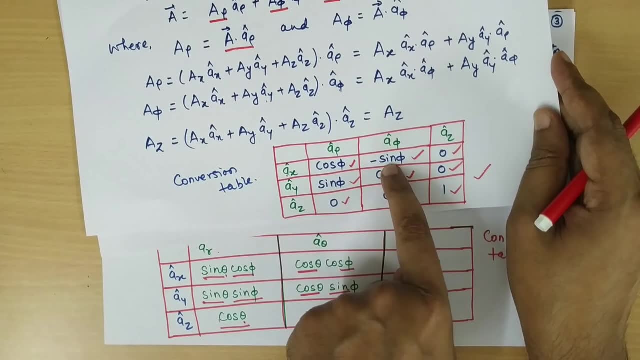 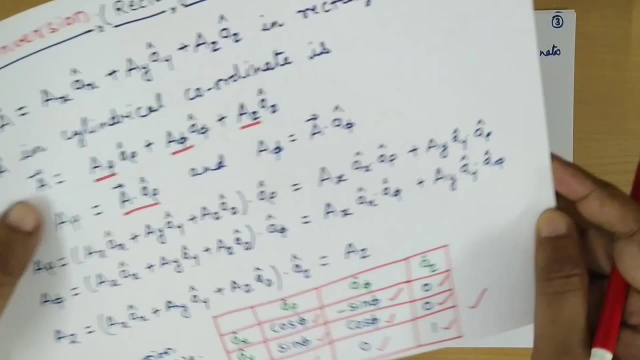 one is minus sine Phi, cos Phi and 0. the logic remains same when we calculate angle between a X and A Phi. that will be 90 plus Phi. so that can be written as minus sine Phi. here also it will be cos Phi and 0. so this is how we can complete. 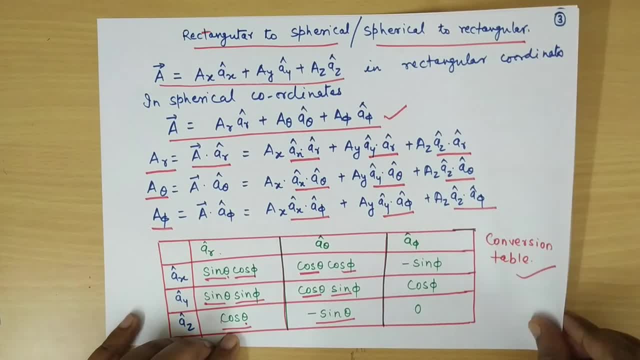 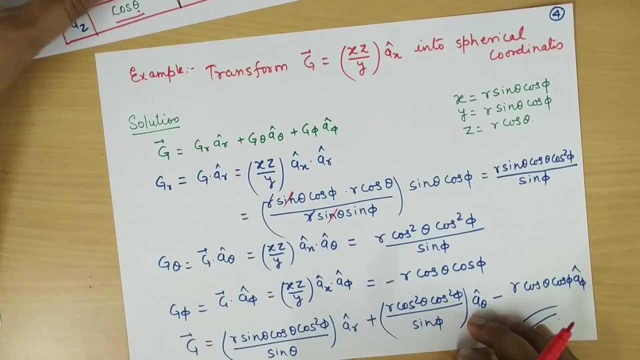 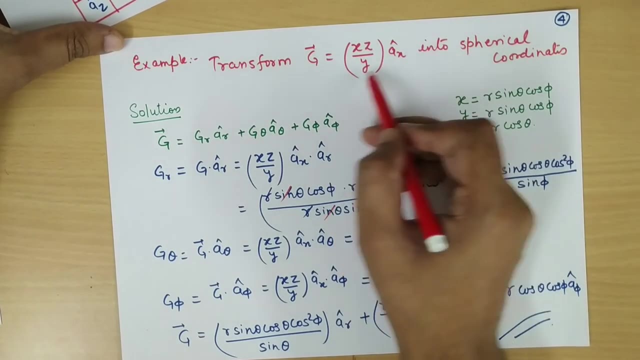 the conversion table and next we'll take one example using this conversion table, we will solve that example. So let us take a vector g, which is xz by y, ax, into a spherical coordinate system. We have to transform this vector into a spherical coordinate system and this vector is only in x direction. 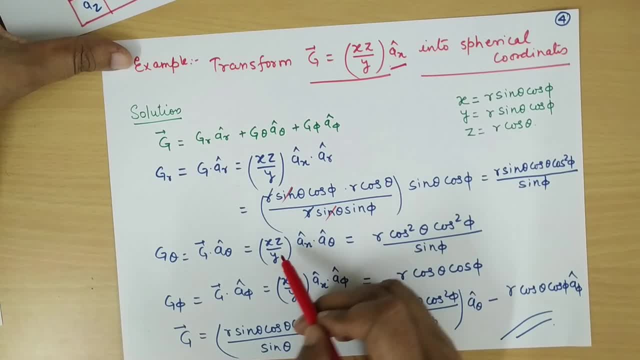 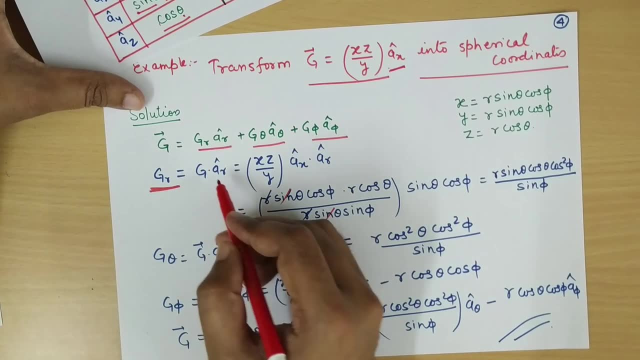 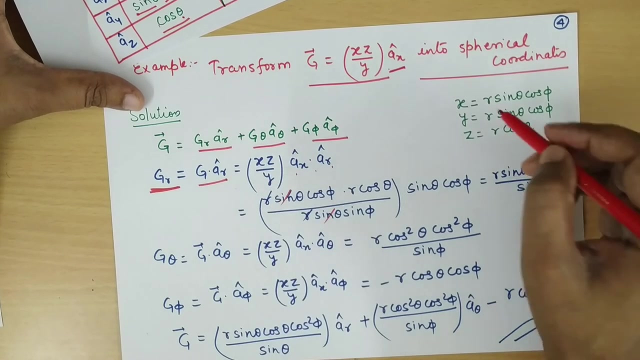 but it will have all the components including gr, g, theta and g far to calculate gr. So these are the three components in a spherical coordinate system to calculate gr. take dot product with ar, so ax, dot, ar, x, z and y can be written from here, which is the formula for converting any point.